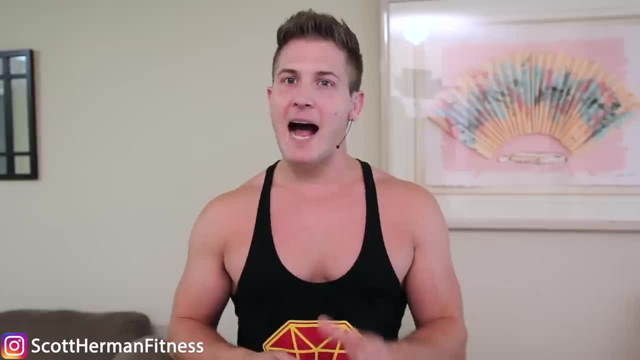 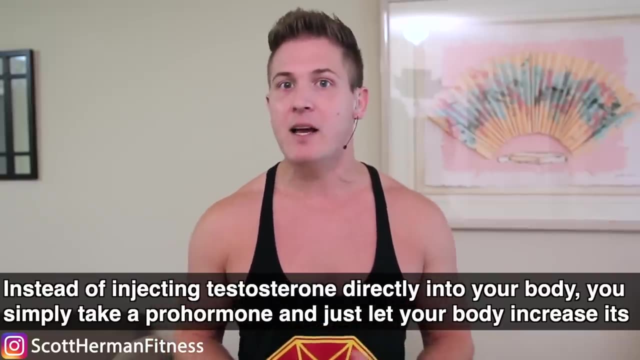 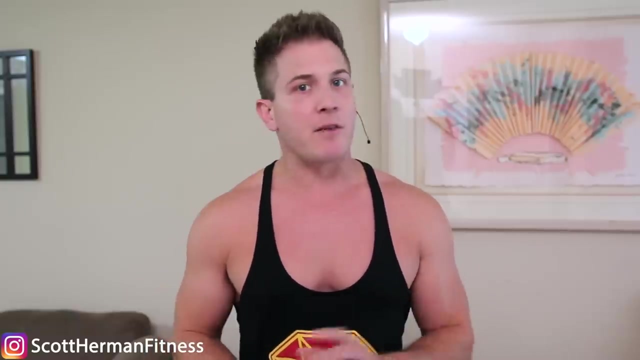 also referred to as natural steroids. But how do pro-hormones compare to actual steroids? Well, in a nutshell, instead of injecting testosterone directly into your body, you simply take a pro-hormone and just let your body increase its production and availability of testosterone. The main 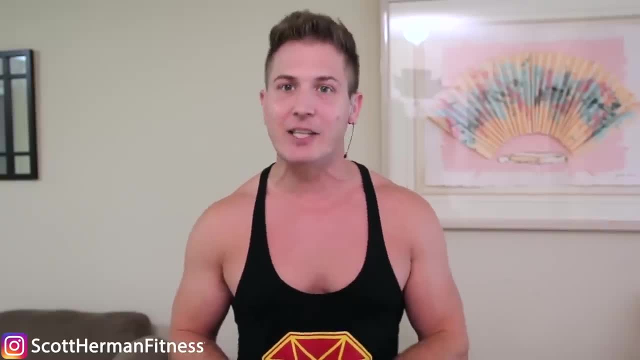 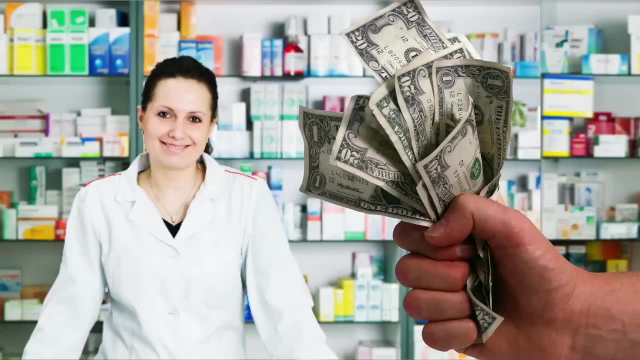 difference is that actual steroids are almost always illegal anywhere you go, whereas pro-hormones are generally legal in most countries and can be purchased over the counter or online. However, most in the world pro-hormones are not, So if you're a pro-hormone, you're going to have to. 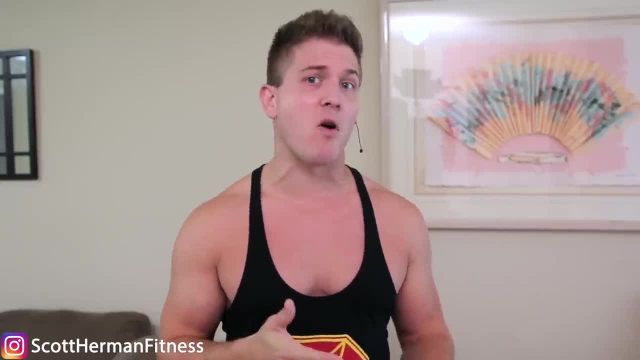 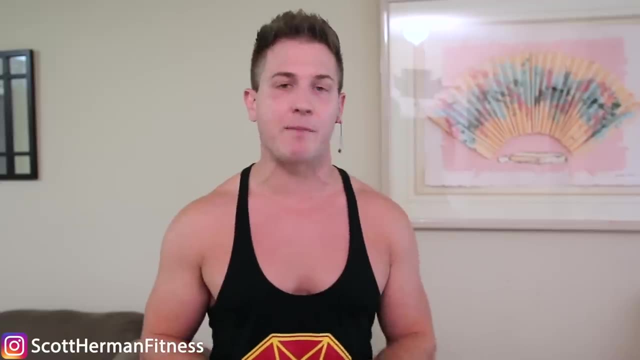 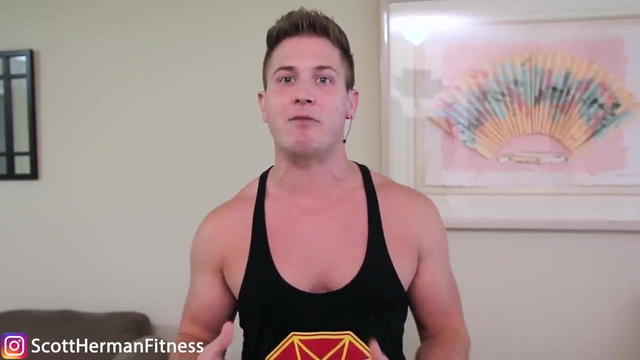 take steroids instead of pro-hormones, because you usually get better results with the same side effects. Therefore, it's safe to say that the only reason why the pro-hormones industry even exists is because steroids are illegal. Pro-hormones are basically a convenient way to get around the 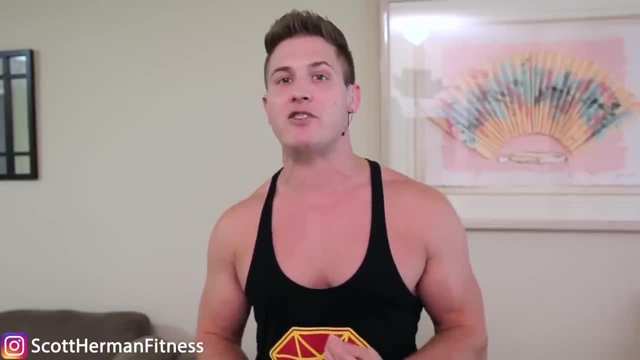 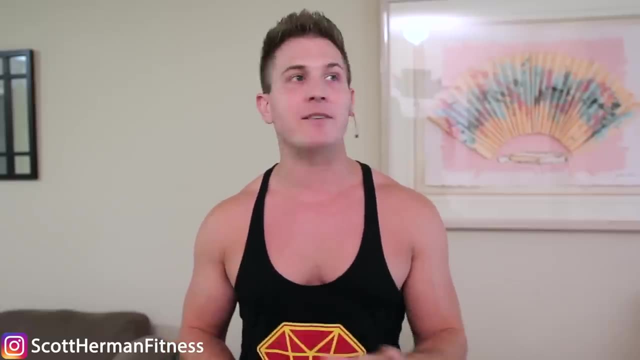 legality of the situation. And to answer the age-old question: are you a natural lifter if you choose to use pro-hormones? No, you most certainly are not. So don't buy into all that BS they're saying out there. If you're a pro-hormone, you're going to have to take steroids instead of 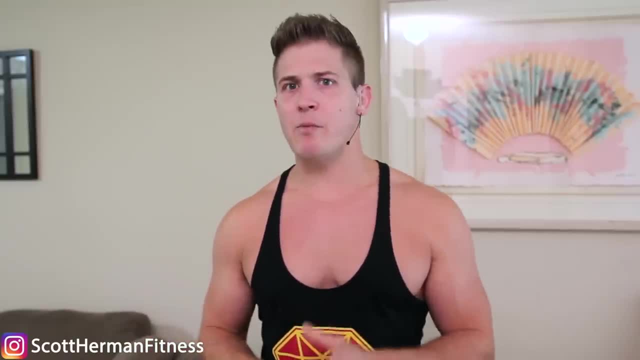 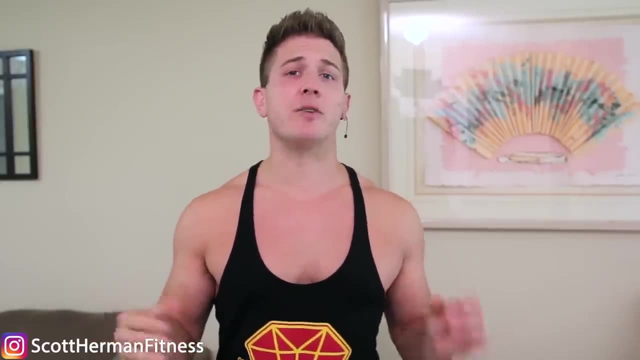 pro-hormones. But let's back up a step real quick. Why would someone choose to get on a pro-hormone cycle? Or, more specifically, what are the potential benefits? Well, the benefits include increased muscle mass, improved physical appearance, superior strength and endurance, better athletic performance. 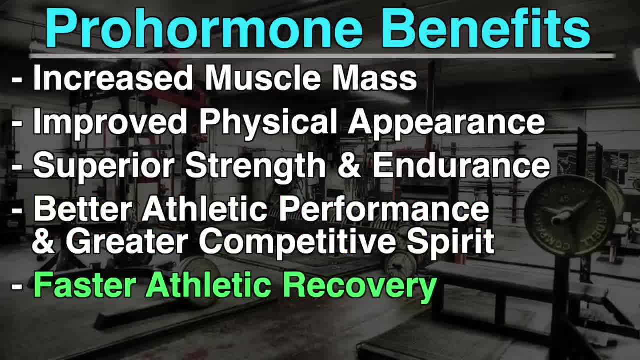 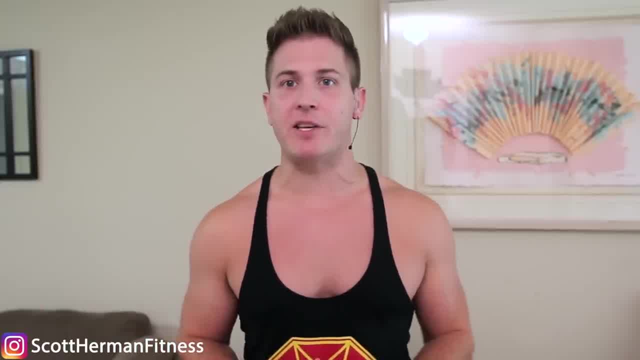 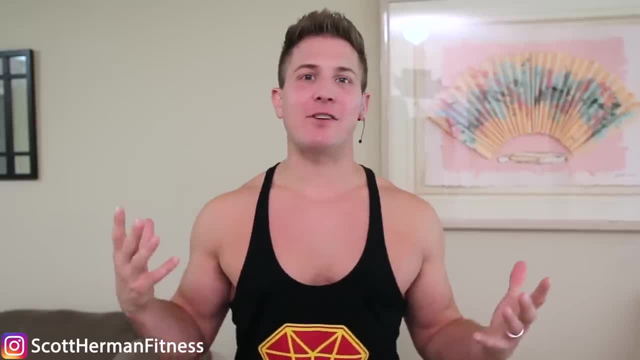 and greater competitive spirit, faster athletic recovery and improved sex drive. Now, guys, take note that these benefits are almost identical to using traditional anabolic steroids, because they are forcefully increasing the production of hormones in your body. So what's the catch? Well, before I dive in, 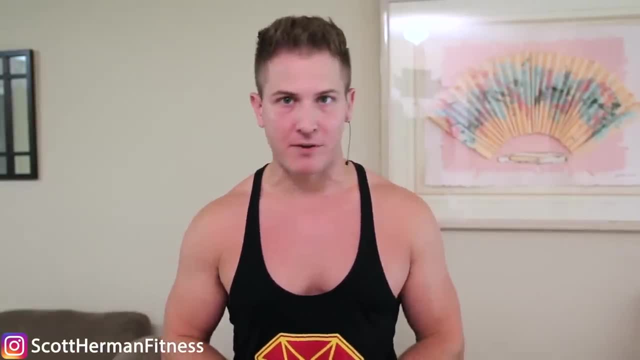 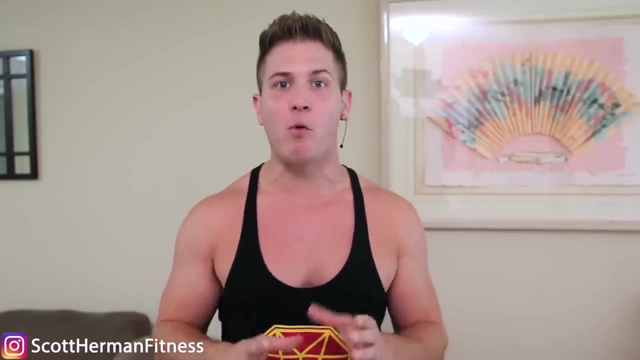 understand that I am not advocating the use of pro-hormones- In fact, I'm highly against the use of any kind of drugs- But in order for you to make informed decisions about what goes into your body, I think it's important for you to. 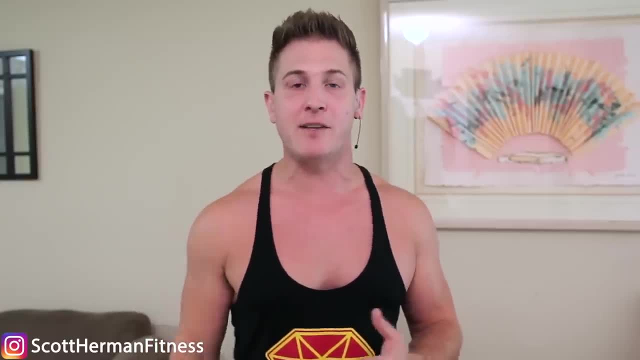 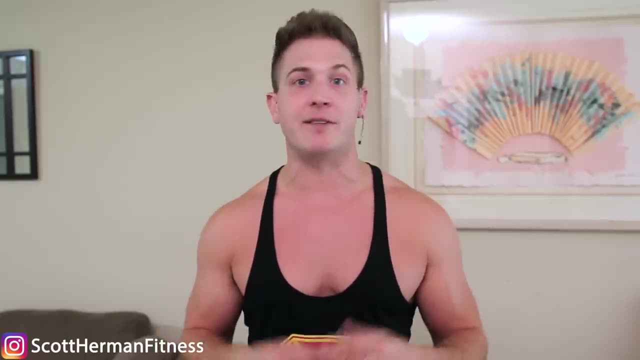 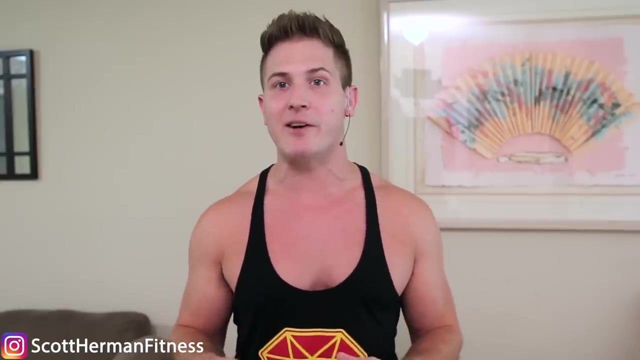 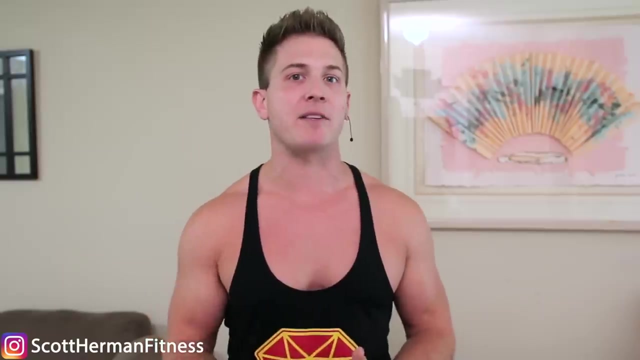 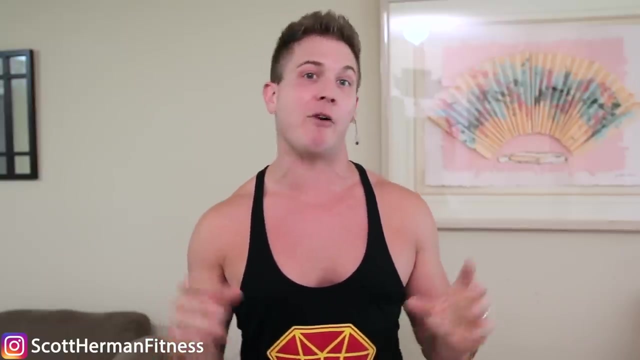 base those decisions off of substance and not just because Scott says drugs are bad. okay, First off, pro-hormones are always deceivingly cheap, And the key word here is deceivingly. Yes, you'll probably be able to get a bottle of your preferred pro-hormone for 30 or 40 bucks, which is enough for one cycle, and you can probably get your entire year's worth of pro-hormones for around 150.. But that's just half of the equation. You actually need to buy three additional components to fortify your health during your cycle and post-cycle. These components are cycle support, liver protection and post-cycle therapy. And then there is the ignorant youth comments of I'm young, I won't have any health issues. 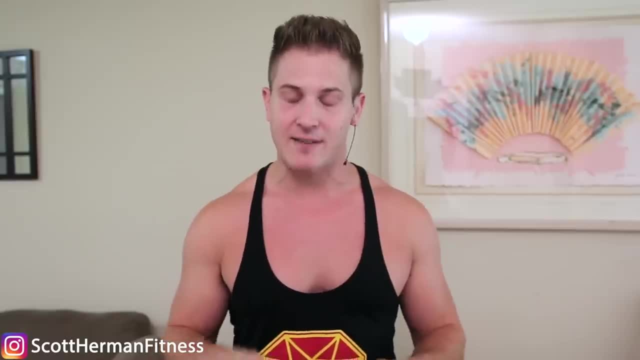 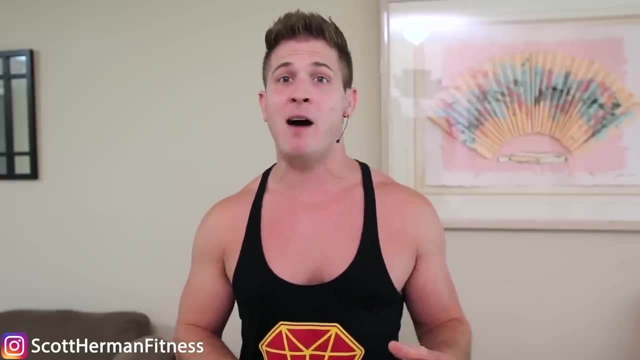 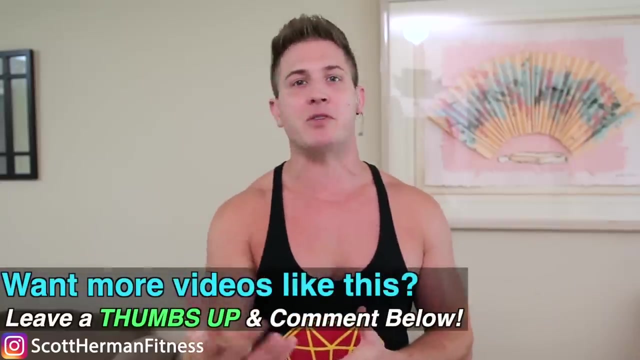 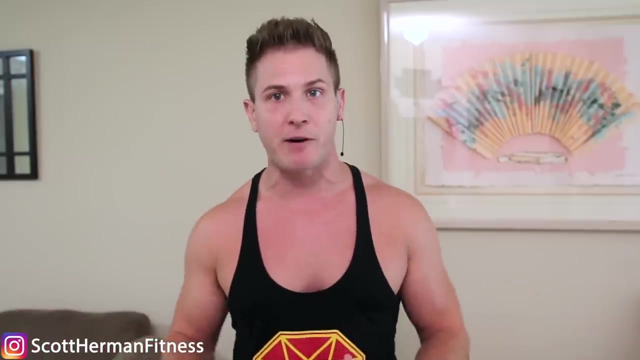 But that is just stupidity at its best, Guys. side effects will occur. It's just a matter of how intense they're going to be. In some individuals they are very mild and in other cases, extremely severe. You'll never know what it will be like for you, Just like those commercials you see on TV for depression medication like Latuda. The entire commercial is basically showing a story of someone being depressed and unable to do anything and then all of a sudden is spending time happily with their friends and family. 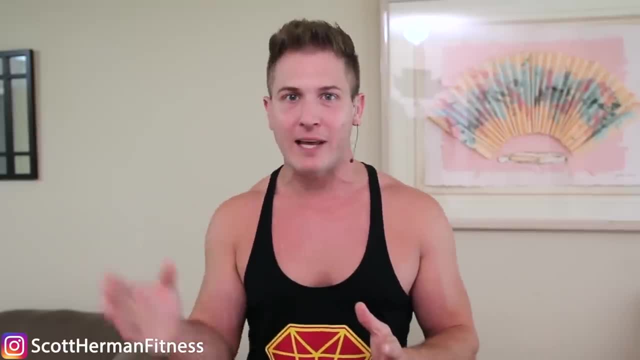 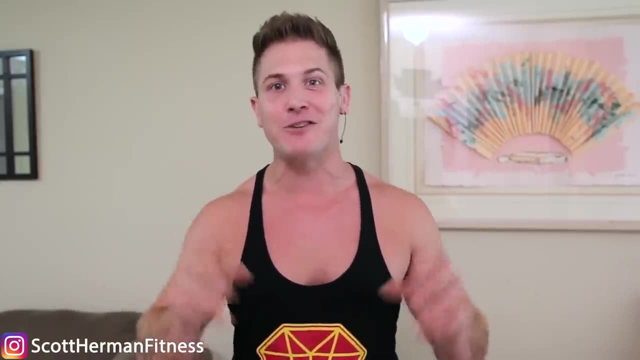 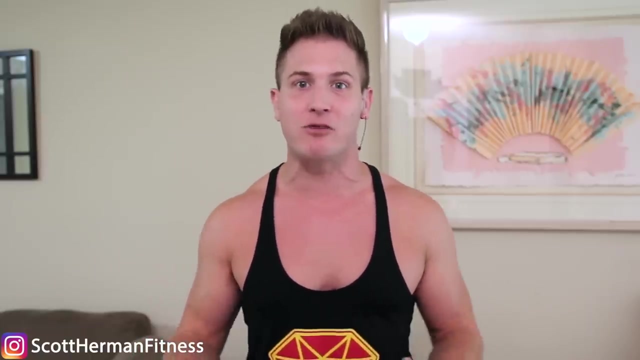 Life is great. but while all this visual stimulation is going on, the narrator of the commercial is saying all the horrible things that can happen to you as potential side effects of taking the drug, One of them even being increased risk of suicidal thoughts, the very thing the drug is supposed to prevent. 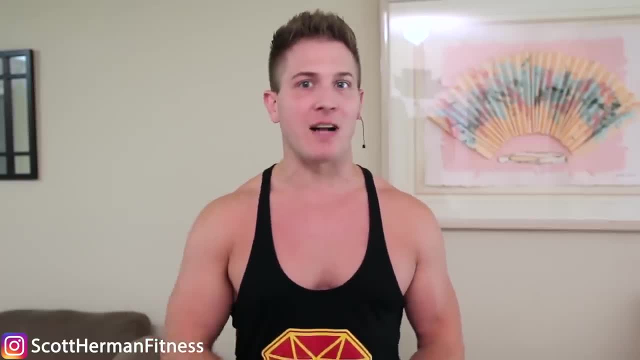 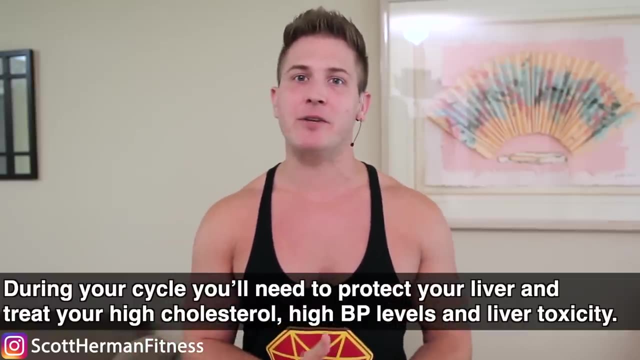 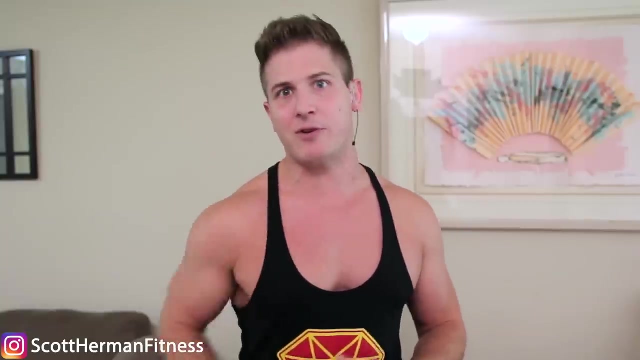 And I'm only saying all this to show you guys, that even legal drugs are not safe, because most people think that anything they can buy legally is safe for them. Now back on track. During your cycle, you'll need to protect yourself. You'll need to protect your liver and treat your high cholesterol, high BP levels and liver toxicity, which is about another $600 per year. 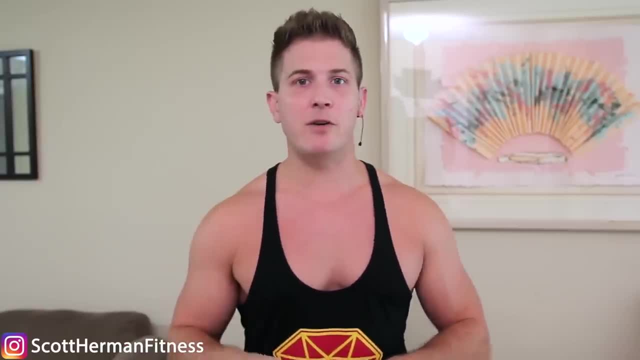 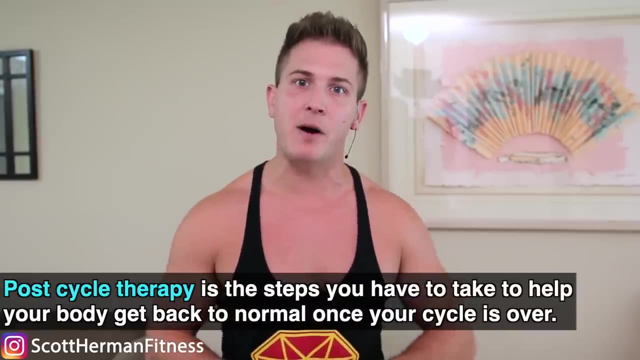 And then you need to take care of your post-cycle therapy Now. for those of you who are not familiar with these types of drugs, which I hope is all of you, post-cycle therapy is the steps you have to take to help your body get back to normal once your cycle is over. 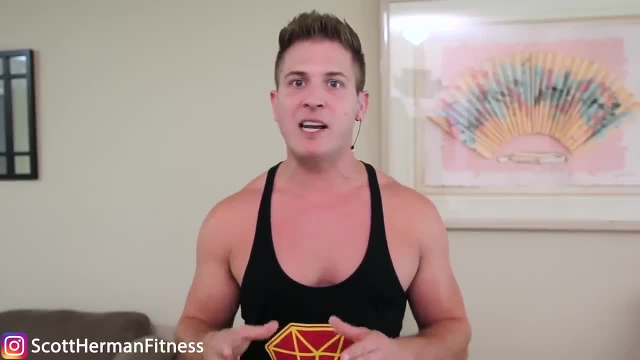 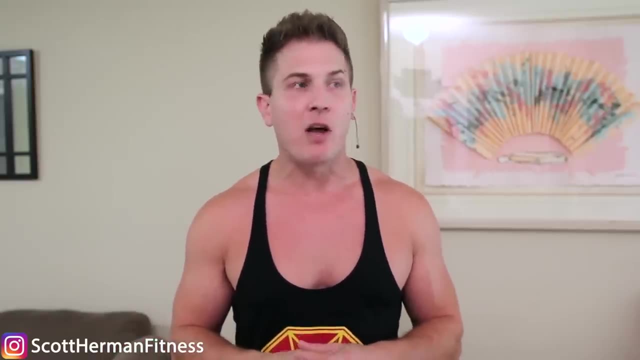 This is because, when you stop using pro-hormones, your body doesn't really know how to maintain normal hormonal levels anymore And therefore your testosterone and estrogen ratios will be kind of out of control, which can lead to some serious side effects. So basically for one month after your cycle and until your body has returned to its normal state, you'll need about another $250 to $400 worth of products, and that leaves us with a grand total close to about $1,000 per year. Now let's get real. I know you all already did the math and are going to say: $1,000 divided by 12 months is only about $83 a month, and I can easily afford that, So why shouldn't I take them? 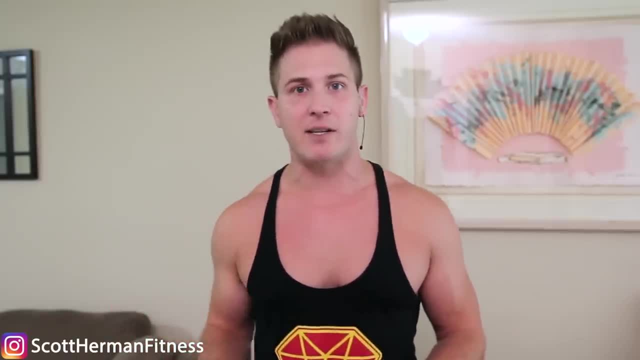 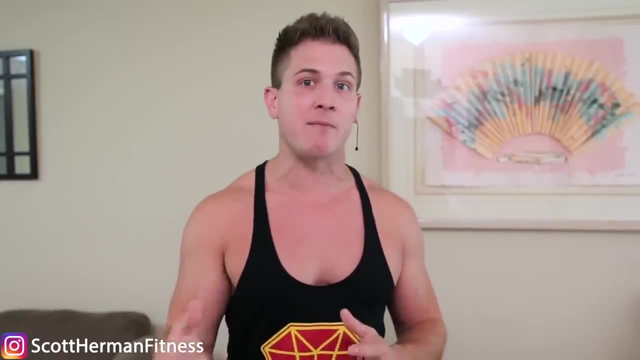 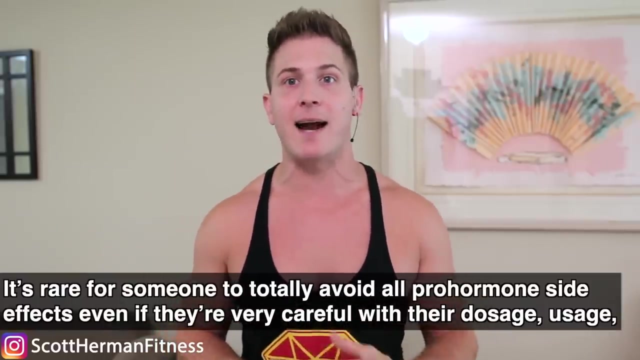 Well, here's why, guys, Pro-hormones, like anabolic steroids, are responsible for a wide range of devastating side effects. Yes, there are ways to avoid these side effects or at least minimize their impact. However, it's rare for someone to totally avoid all pro-hormone side effects, even if they're very careful with their dosage, usage and post-cycle therapy. 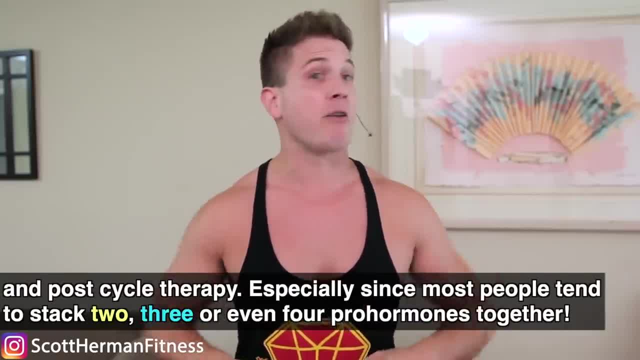 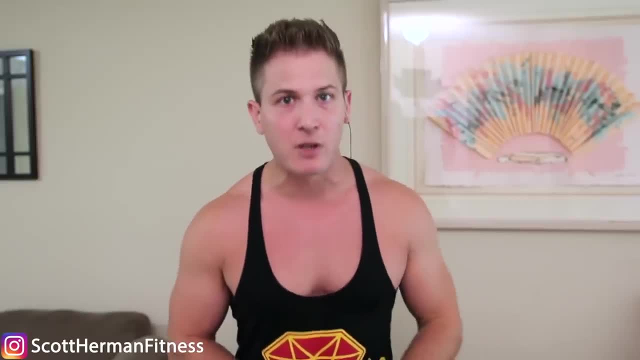 And if you're one of these people, you're not going to avoid them. Ridiculously ignorant people who are going to comment below. if you do it right, You'll be okay. I'd like for you to just to take a second and repeatedly punch yourself in the face. 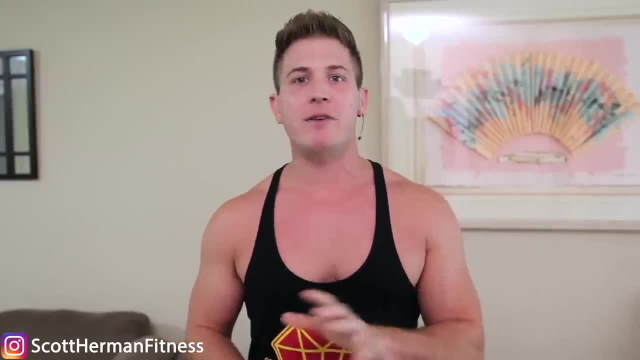 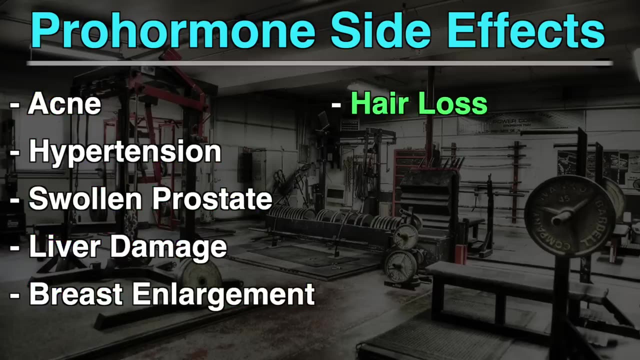 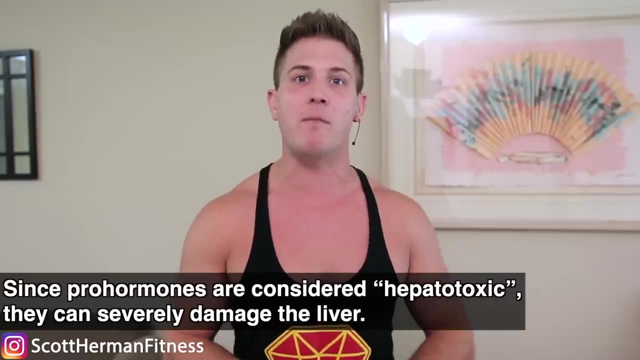 Until you knock some common sense into your brain. now here are the side effects while cycling on and off pro hormones: acne, hypertension, swollen prostate, liver damage, breast enlargement, hair loss, more facial hair growth, deeper voice, headaches, dizziness and nausea. and, Worst of all, since pro hormones are considered hepatotoxic, They can severely damage the liver. 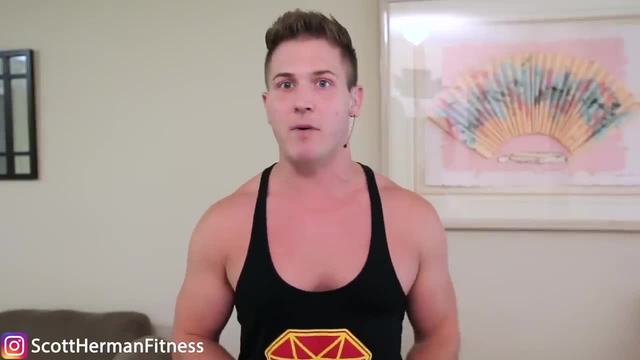 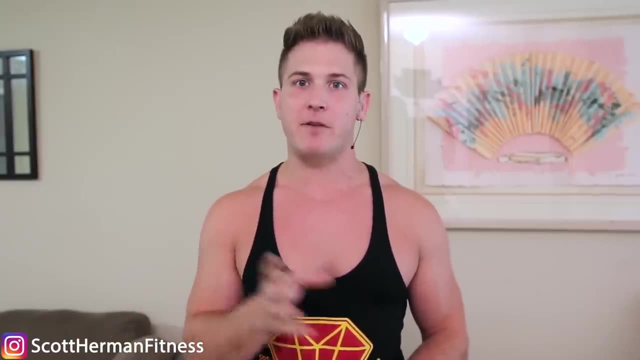 That's why it's recommended that you cycle on and off pro hormones. Alright. so the final verdict, guys, Is it worth investing in pro hormones? Well, carefully think about the following points before making a decision. Number one: very few people actually recommend taking pro hormones. 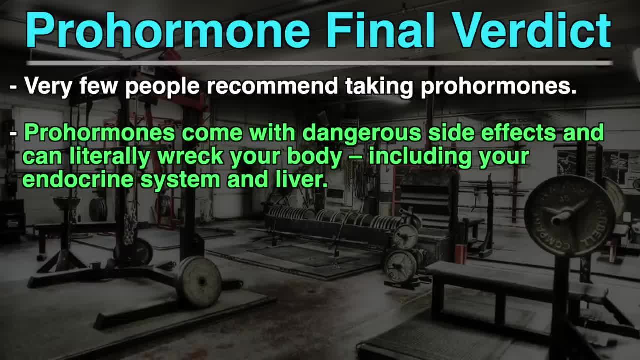 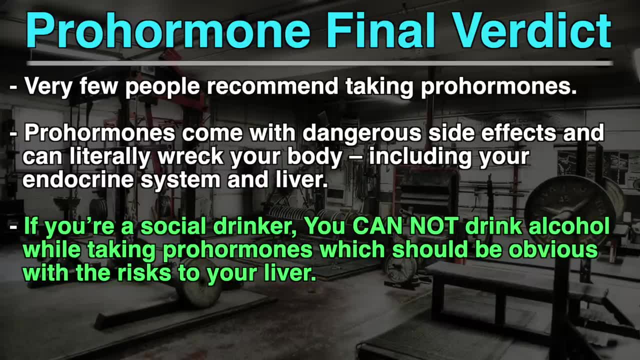 Number two: pro hormones come with dangerous side effects and can literally wreck your body, including your endogenous Ocarina system and liver. and number three: if you're a social drinker, You cannot drink alcohol while taking pro hormones- which should be obvious- with the risk to your liver. 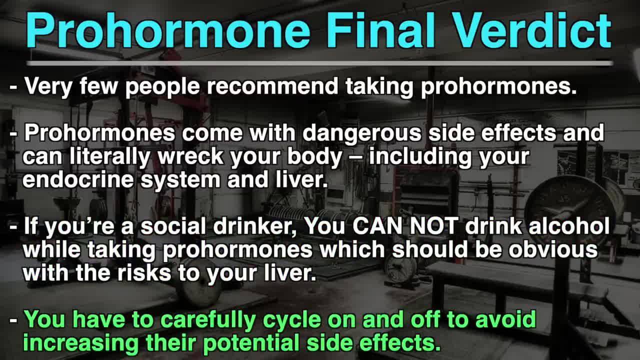 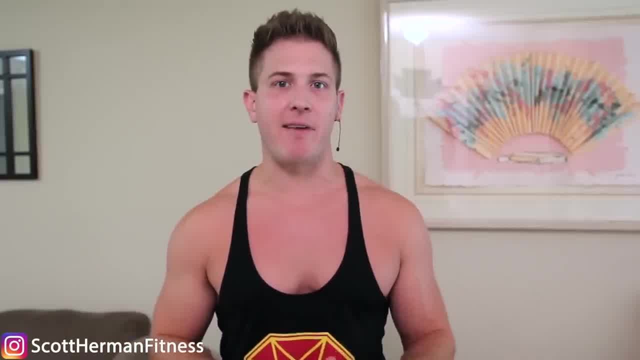 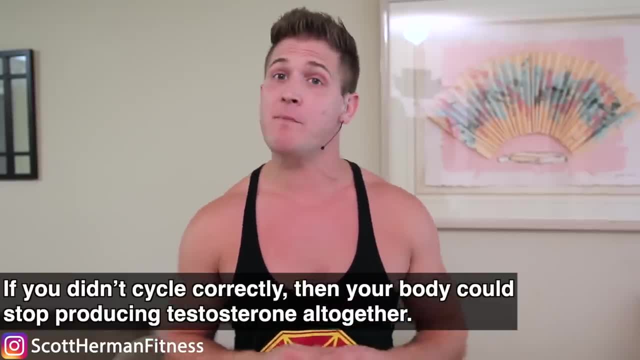 And lastly, you have to carefully cycle on and off to avoid increasing their potential side effects. But even if you could get around all of that, You can never get around the fact that pro hormone induced results typically do not last. Also, if you didn't cycle correctly, then your body could stop producing testosterone altogether. 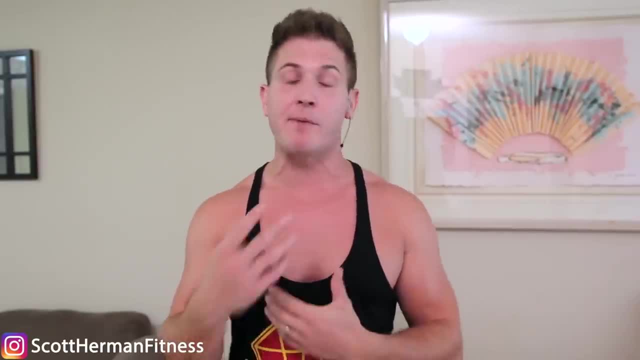 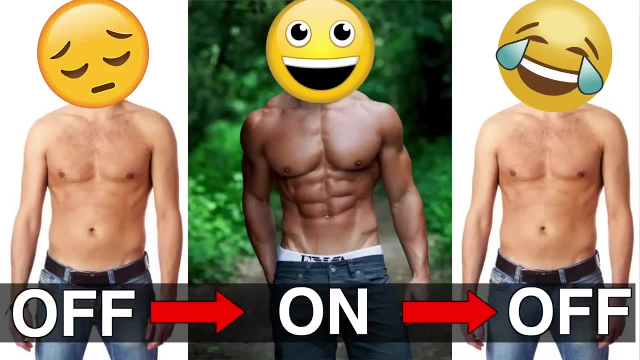 Which means you could be much worse off than when you were before jumping on the pro hormones. And what about the gains you did make? well, 80 to 100 percent of your gains will most likely be lost, since the only Reason they occurred in the first place was the pro hormones. 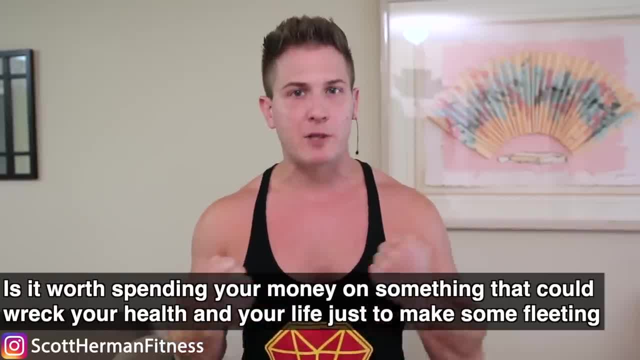 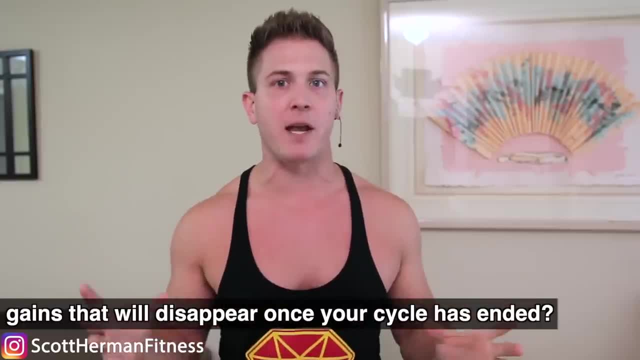 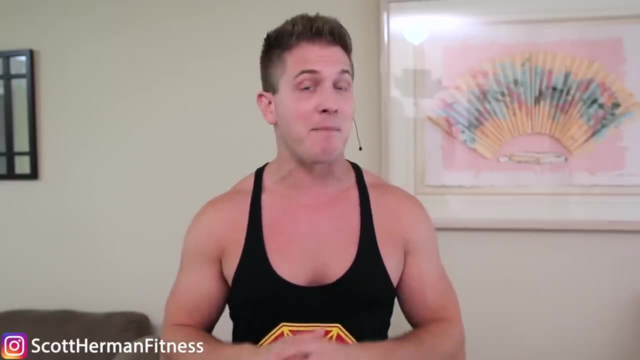 So ask yourself the following question: Is it worth spending your money on something that could wreck your health and your life Just to make some fleeting gains that will disappear once your cycle has ended? Well, let's talk about the last piece of this equation Before we end the video. as I'm sure you've already guessed, many physique athletes and fitness competitors tend to think that the pro hormones 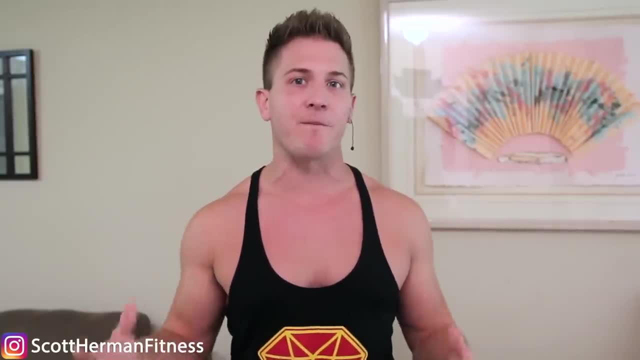 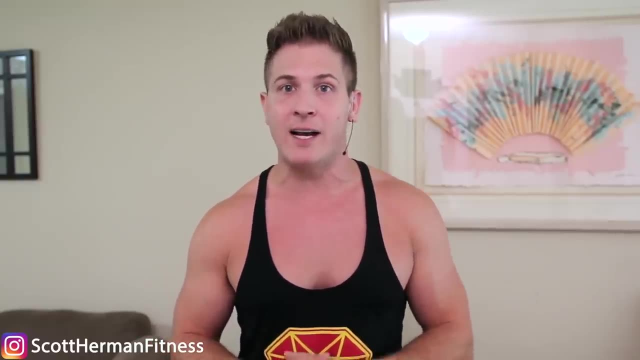 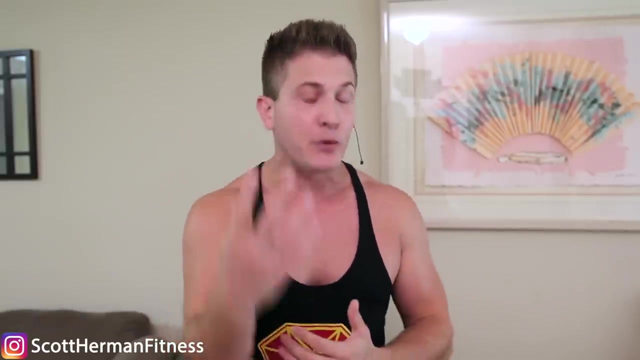 Benefits outweigh their side effects, Especially since their fame and income depends on it, and as much as you don't want to hear it, a lot of your favorite natural athletes you follow online are taking low dosages of drugs to maintain their lean and Natural look all year round and to fool you into buying their programs and invest in their careers. 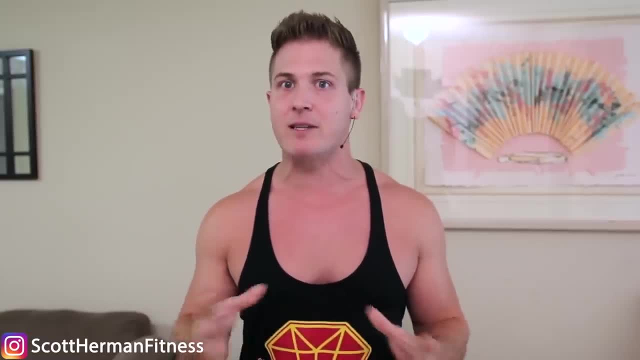 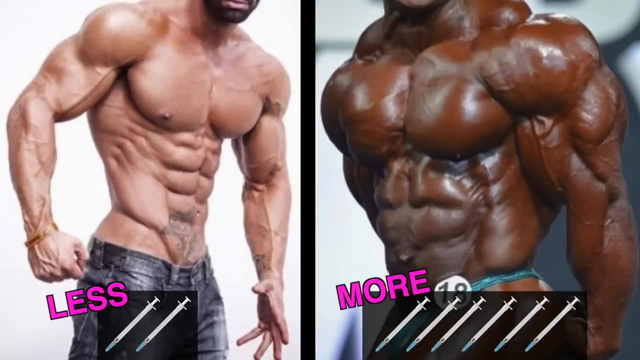 It's like most people Nowadays don't realize that steroids come in many different forms and they do not all lead to that freakishly bulky physique We've come to perceive as the steroid physique. So if you're looking into pro hormones or someone like this is talking about pro hormones- 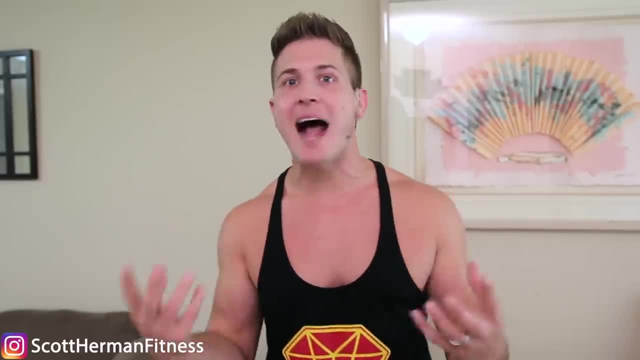 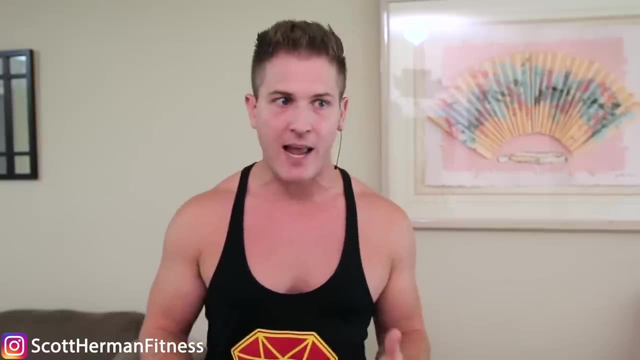 And how they're not like steroids and how they're. they're more of a natural solution to making gains And they're easy to do and to follow. as you've just seen from this video, They're not. they actually have quite a bit of maintenance With them. you have to cycle on and off this post cycle therapy. 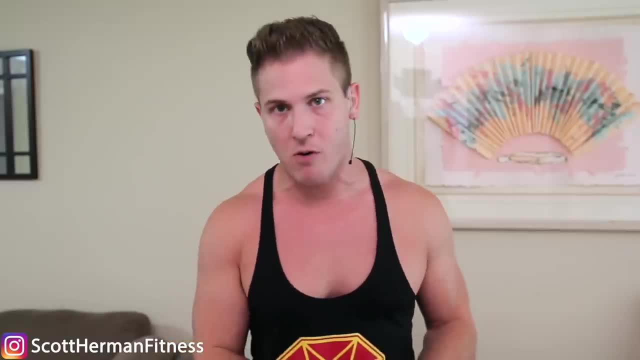 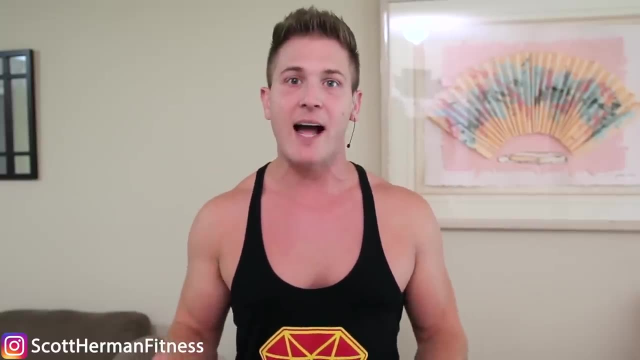 There are some serious risks involved with doing pro hormones. So if you're looking into them and you think it's a walk in the park, you have to understand that it's not. and, guys, Fitness isn't hot. all you need to succeed is consistency with your training and your diet.